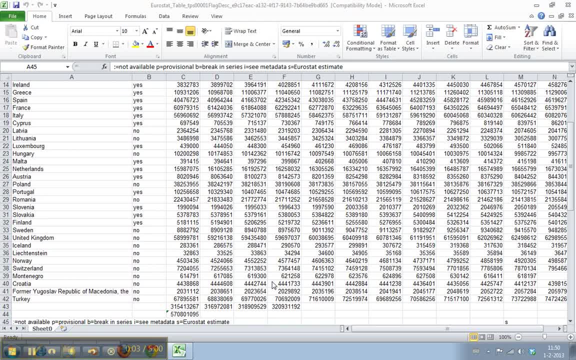 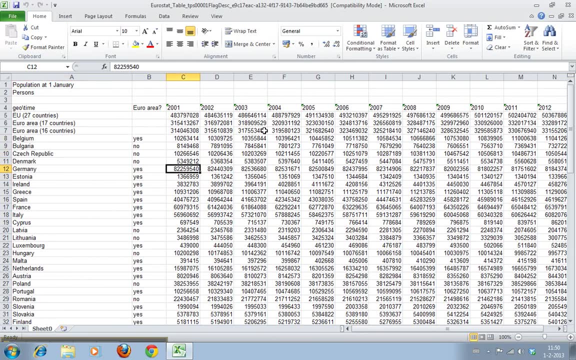 Welcome to WorkSmarterTV. I am Maarten and in this video I will show you how to calculate percentages. We have our big data set of European Union countries with population data for the years 2001 until 2012.. Now this is all a big bunch of numbers that's pretty hard to 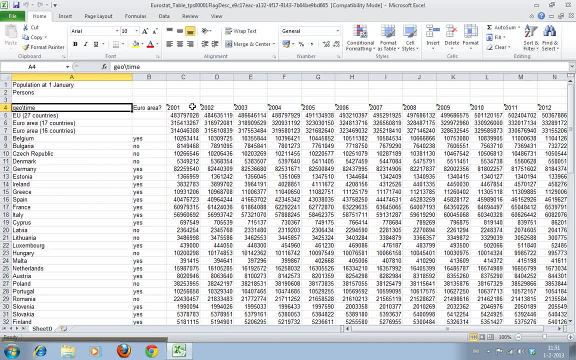 actually get something out of. So a very good way to interpret this is to actually calculate the percentage increase from year to year. Well, we'll start by. the easiest way to do this with big data sets is by just creating another worksheet where we will then have in this exact same cell, 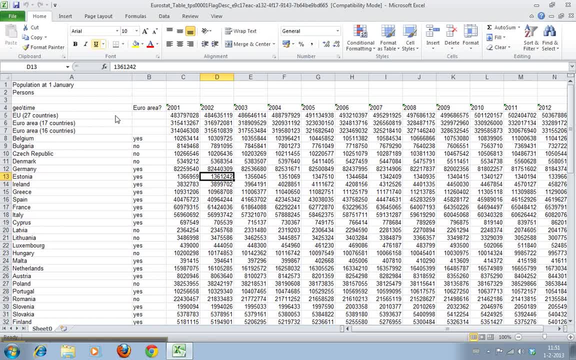 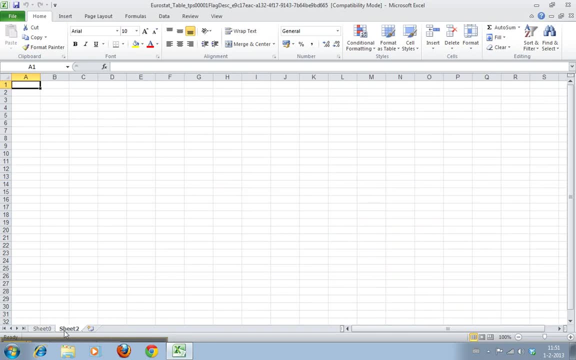 configuration. So this is a column with the names and this is a row with the year dates and we can just fill that with a with handy formulas. So we'll start with creating a new worksheet. You do this here: insert worksheet and we have it. sheet two: Let's just rename this one. 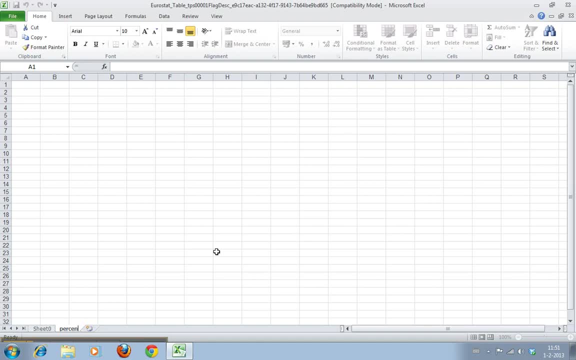 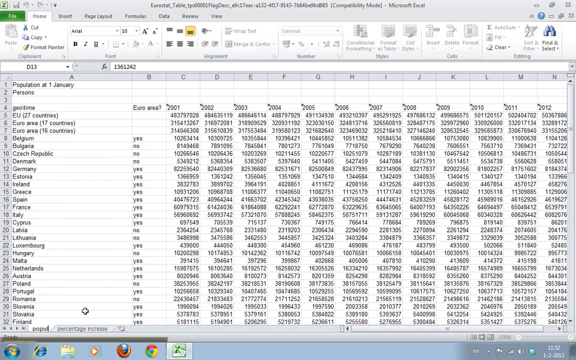 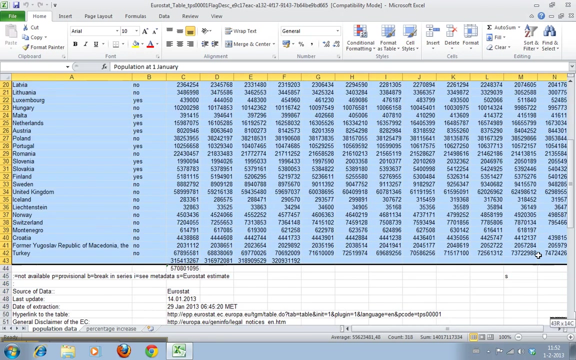 You can double click it and rename it: percentage increase. So we can always- and this is population data- You can just double click it and then click somewhere else and it's done. First, we start by copying everything from the first few rows until here: Copy. 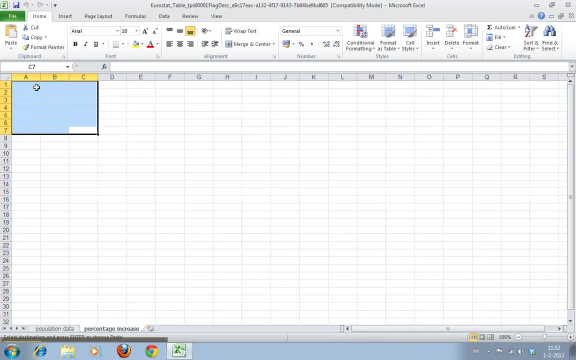 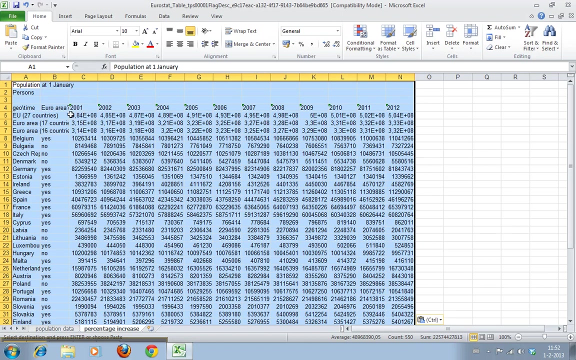 right mouse button, copy, and then we go to the very first cell and we click paste. Well, yeah, this is what we want. and now we get some funny stuff here. It says 4.84 e, point. It's plus eight. What it's saying is it says I've got eight more digits and I can't, I don't have. 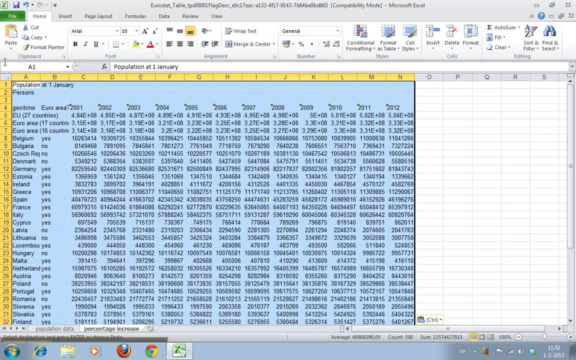 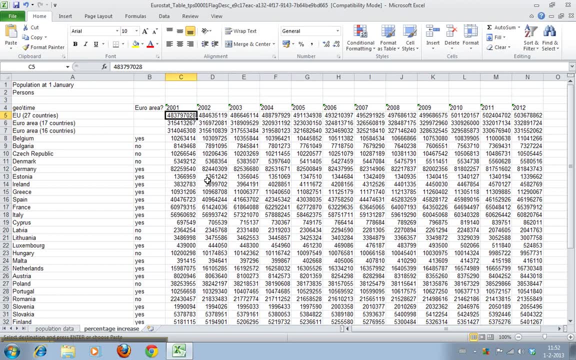 any space for them. So it displays it like this: If we select all this and we double click here, it just adjusts the space and then we have regular numbers again. But we don't want these numbers. We want to calculate the percentage increases in these cells. So what we'll do is we'll just empty. 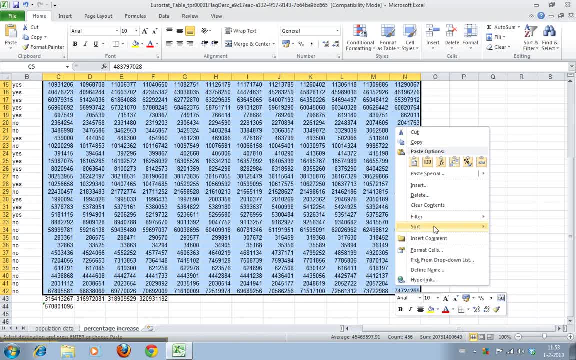 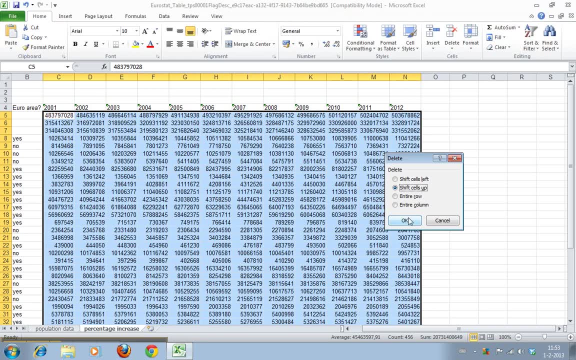 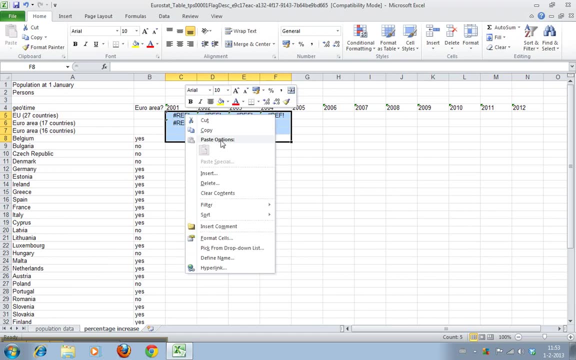 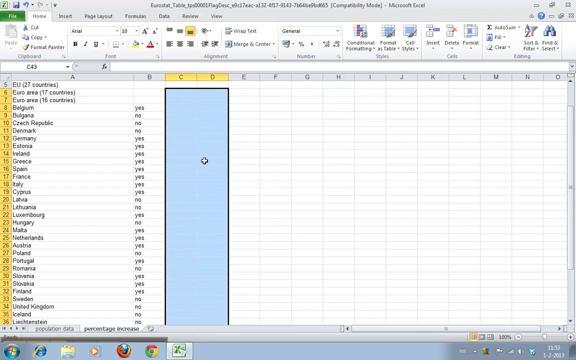 them. Oh, delete, Yeah, shift. so this can be relevant, but it's not now, because it doesn't matter where they go, It's just make them empty. Ah, still trying to calculate stuff here. Don't calculate stuff, Get it out. Oh yeah, that's what. the cells here were shifted over there. Um, okay, so how do we calculate the? 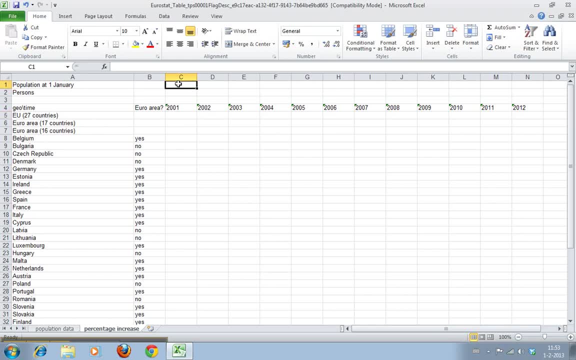 percentage If this. let's just do a trial or anything here. This is 100 and this is 110.. Oh, 10.. If we want to calculate the percentage, it is the new value minus the old value, It's 10.. Then we put brackets around it. 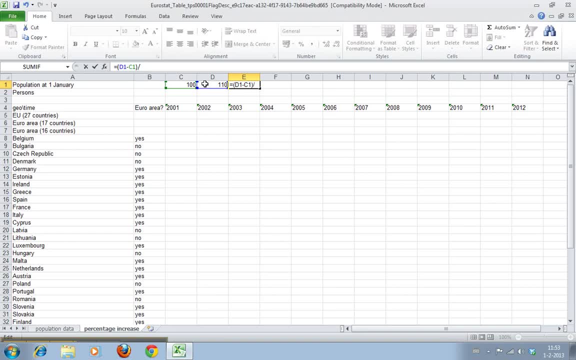 And then we say: divide it by the old value, By the old value 0.1, which is 10 percent, and then we add this one and it says 10 percent. That's how basically a percentage works. So now we do this here, So this is the old value. 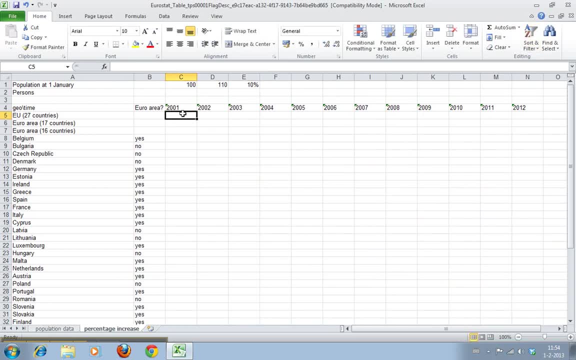 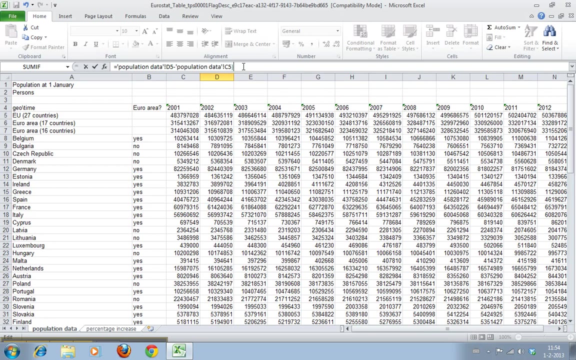 And we're gonna: no, let's do. sorry, let's just do that because this is basically the our. the 2001 value will be our 100.. Is this minus that one? Put brackets around it because otherwise it will just divide the second data, the second to the c5 divided by this one, and we don't want that. and now we create a percentage in it. 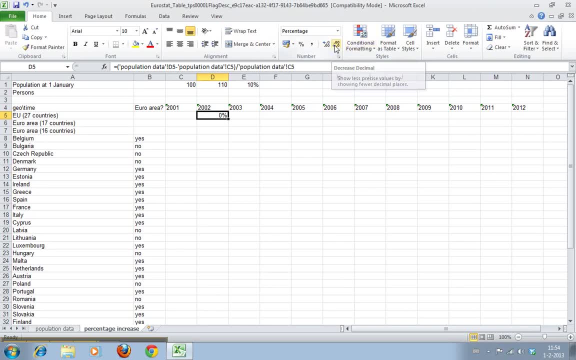 and that's zero because it's very small, so we move the comma. sorry, uh, of course we can't move it that way, and so it's increased for all european countries. european union countries from 2001 to 2002 is 0.17%. 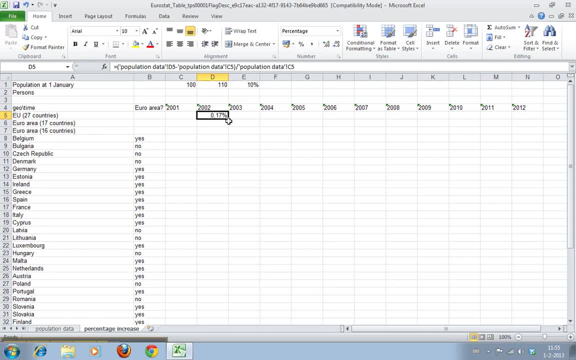 in part two of this video, i will show you how to use this formula and copy. copy it to the entire cell. so watch out for part two. i hope you found this video helpful. if you have any questions, you can leave them in the comments. um, you can subscribe to my youtube.